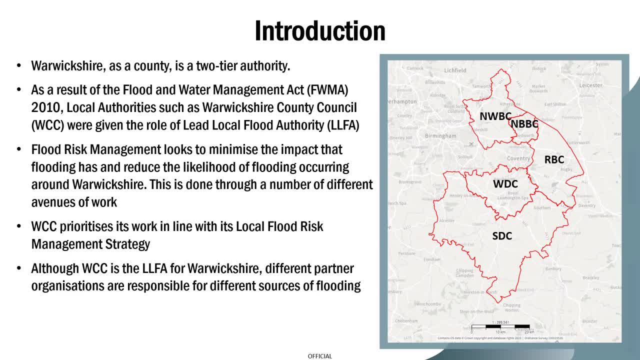 that flooding has on communities and reducing the likelihood of flooding occurring around Warwickshire. This is done through a number of different avenues of work, such as our statutory planning and consenting role, our involvement in investigation and enforcement work and our work in communities, working with flood action groups and working to deliver capital schemes. 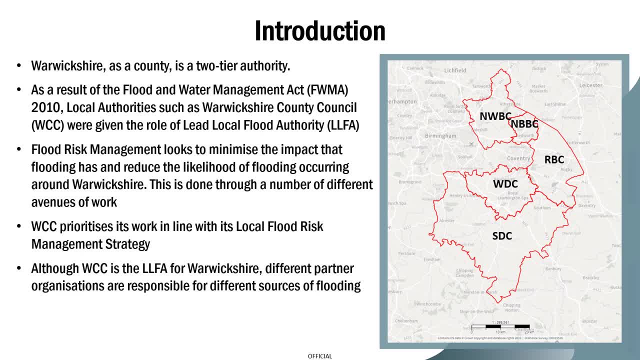 Due to the volume of work the team has, we prioritise our work in line with our local flood response strategy, which is available on our website, but please note we are carrying out an update on this. The hierarchy is as follows: So number one: flooding that poses a threat to. 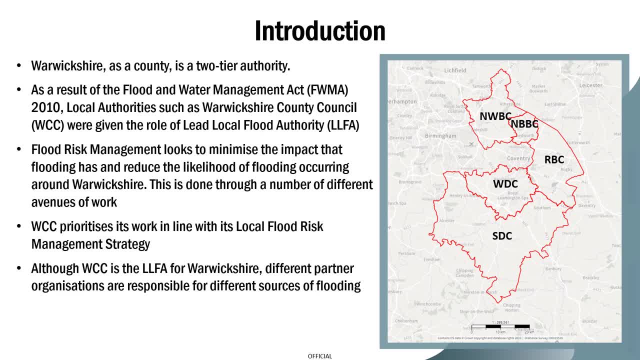 the safety of the public or may directly result in serious injury or death. Number two: five or more residential properties internally flooded. Number three: two or more commercial properties internally flooded. Number four: one or more piece of critical infrastructure affected that impacts on the wider area. Number five: flooding that places vulnerable individuals or vulnerable. 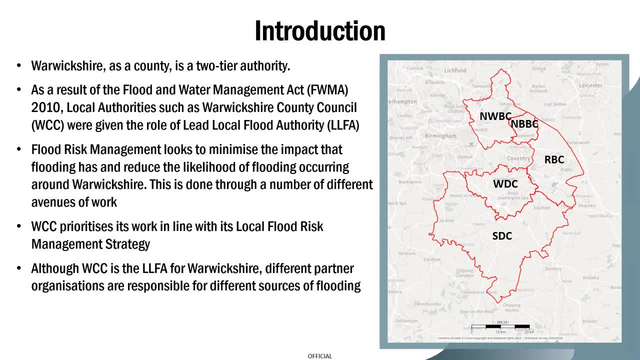 communities at risk, for example, hospitals, inner wheel available housing, nursing homes and schools. Number six, where one or more residential property has flooded internally on the same source on five or more occasions the last five years. It's also important to note that, although Warwickshire County Council are the 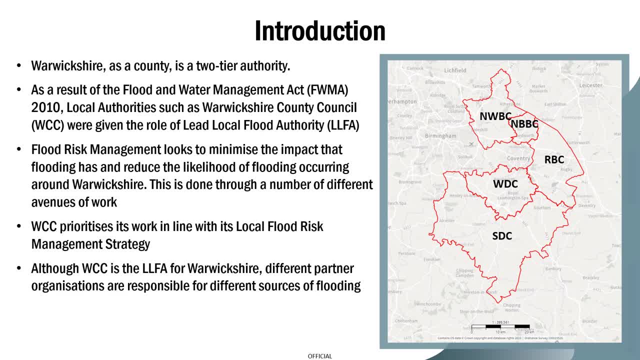 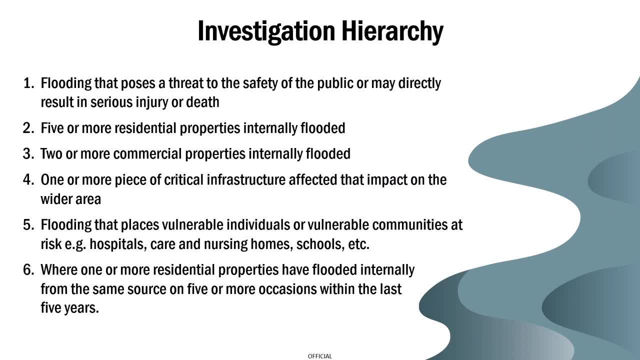 lead local flood authority for Warwickshire. different partner organisations are responsible for different sources of flooding which we will expand on later. As mentioned in the previous slide, due to the volume of work the team has, we prioritise our work in line with our local 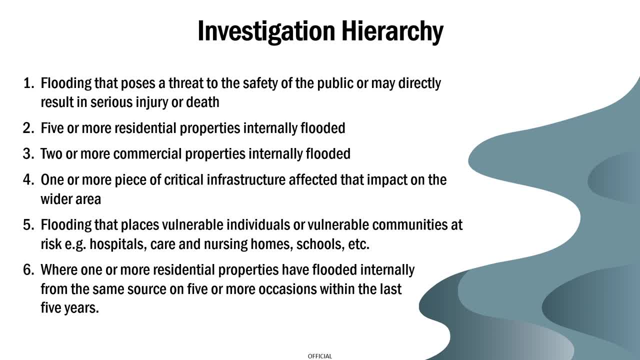 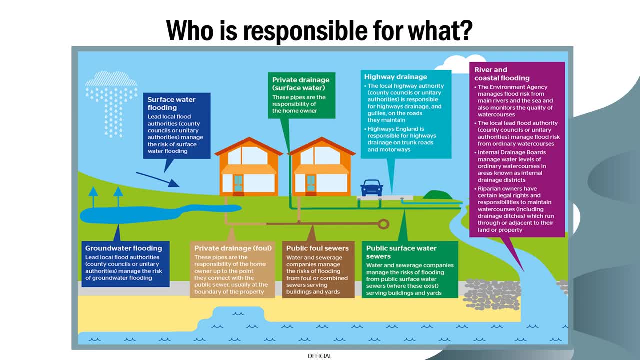 flood management strategy. The investigation hierarchy has been detailed on this slide. So which organisation is responsible for what? As you can see, our team are responsible for surface water, groundwater and river flooding from all new water courses. Any form of private drainage, whether it be surface water or foul, would be a responsibility. 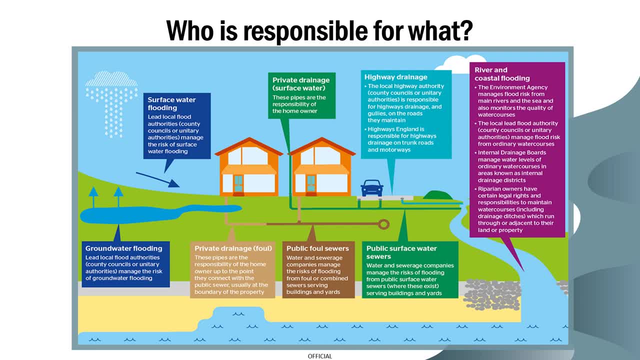 of the homeowner up to the point where the connection is made with a public sewer. Public drainage, whether it be surface water or foul sewers, would be the responsibility of the water and sewage companies and all the others involved. Let's go on to the next slide. 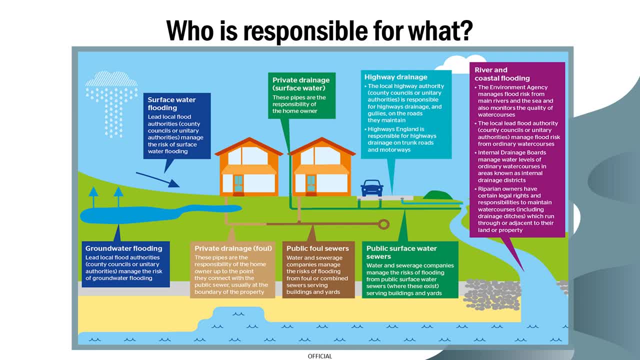 highway drainage is the responsibility of the local highway authority for the roads that they maintain. for the majority of warwickshire. public drainage, excluding highway drainage, would be the responsibility of seven train water. as i mentioned earlier, the lead local flood authority is responsible for groundwater, surface water and river flooding from northern watercourse. 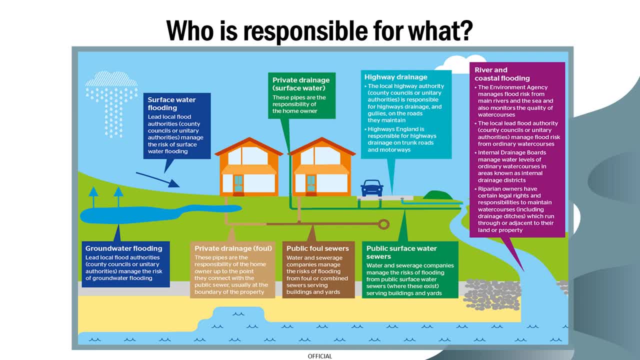 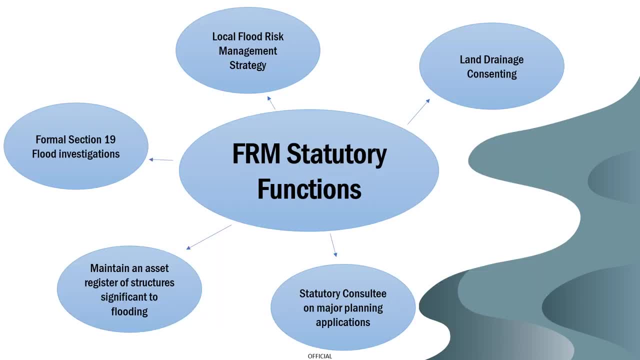 any flooding occurring from any of these sources will be investigated in line with that investigation hierarchy, which is highlighted on the previous slide. i won't spend too long on this slide, but here we are highlighting all of the statutory functions we hold in the team. these include ordinary water sports, land drainage, consenting being a statutory 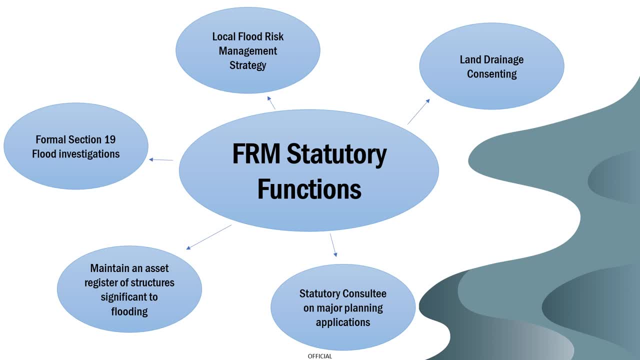 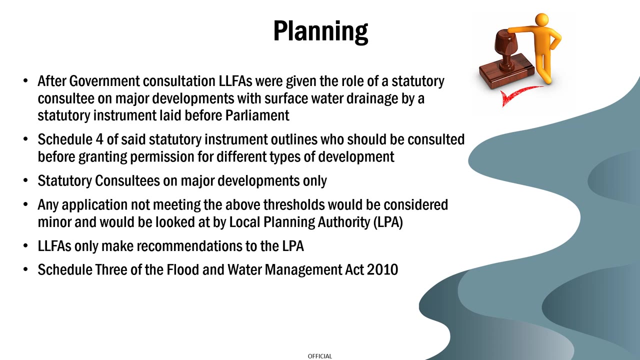 consultee on major planning applications. formal section 19: flood investigations, maintaining an asset register of structures significant to flood risk and having a local management strategy in place. so let's have a look at our first statutory role, which is the assessment of major planning applications. our first 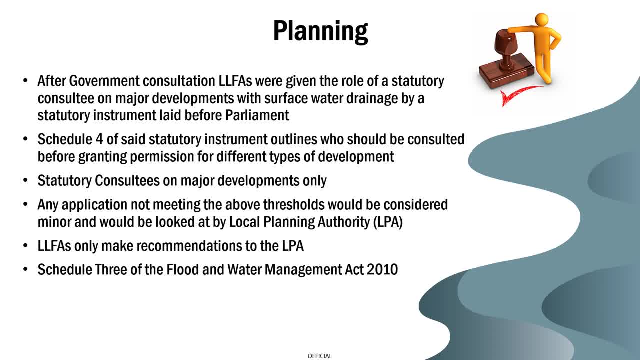 the government consultation on the 15th of april 2015, lead local flood authorities were given the role of a statutory consultee on major developments with surface water drainage by a statutory instrument laid before parliament on the 24th of march 2015.. schedule 4 of said statutory instrument. 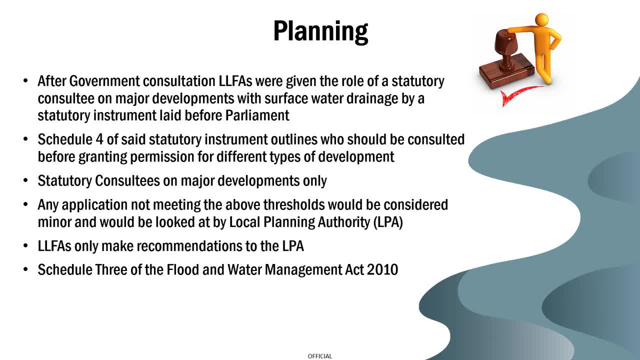 outlines who should be consulted before granting permission for different types of development. these could include the environment agency, canada rivers trust, natural england and seven train water, for example, lead local flood authorities. only statutory consultees are major developments. major development thresholds consist of developments for 10 or more dwellings, one hectare or more in floor space, waste. 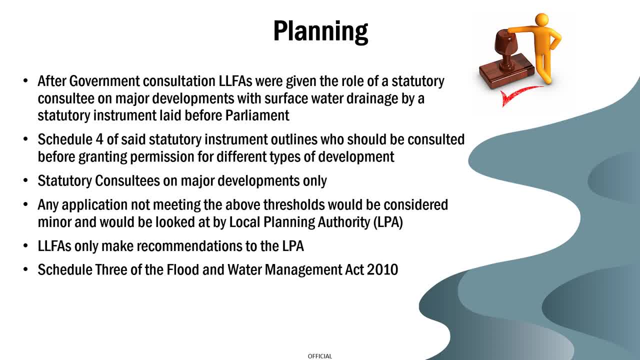 developments, mining and workings of materials. any application not meeting the above thresholds would be considered a minor development and would be looked at by the local planning authority and the district and borough councils lead. local flood flood authorities only make recommendations to the local planning authority but at local planning authorities can ultimately choose to. 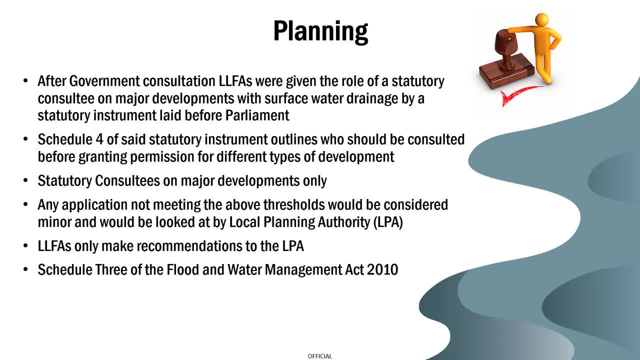 choose whether or not to take on board this recommendation. by the 10th of january 2023, defra published the review for implementation of schedule 3 to the flood and water management act 2010.. this recommended recommended implementation of schedule 3, which the government has accepted. 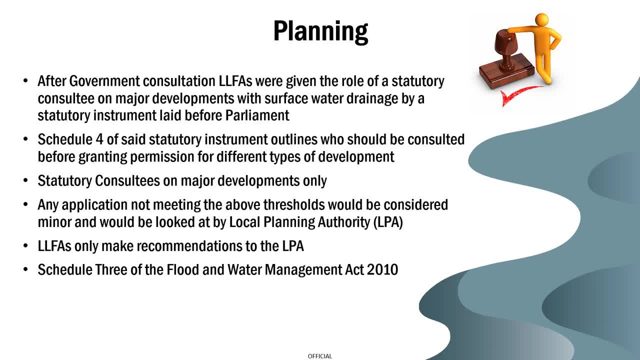 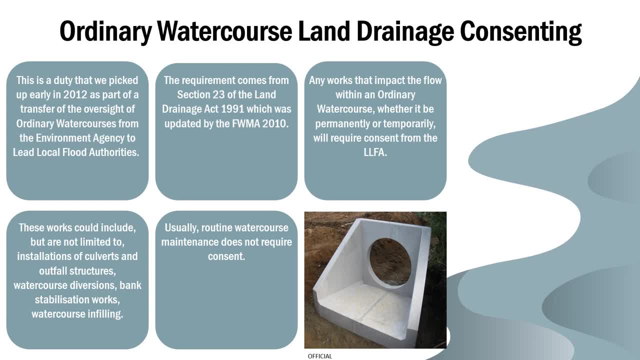 warwick county council will shortly be taken on the role of suds approval body. in the future, all new water sports- and andrea sending is a juice that llfa is picked up in early in 2012 as part of a transfer of the oversight of ordinary water courses. 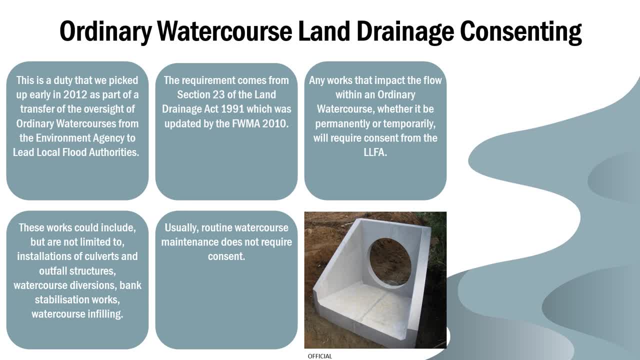 from the environment agency to lead local flood authorities or internal drainage boards. the requirement to assess land range consent applications comes from section 23 of the land drainage act, which is updated by the flood and water management act 2010.. broadly speaking, any words that impact the flow within the ordinary water course, whether it be permanently or 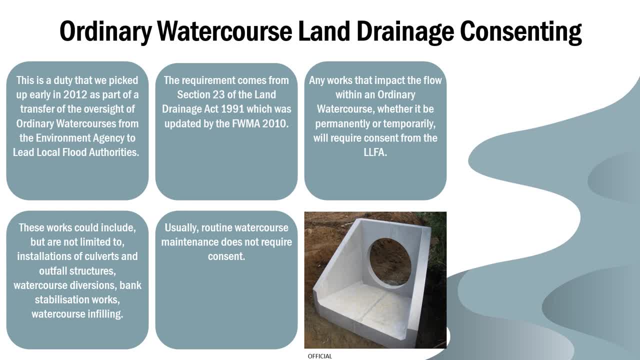 temporarily will require consent from the lfa. by the way, there are five different version of the law regarding the flow of water, including the flow rate, the process of the flow rate, and it also includes the length of the flow and water content. each work can be interpreted together with a specific type of water and 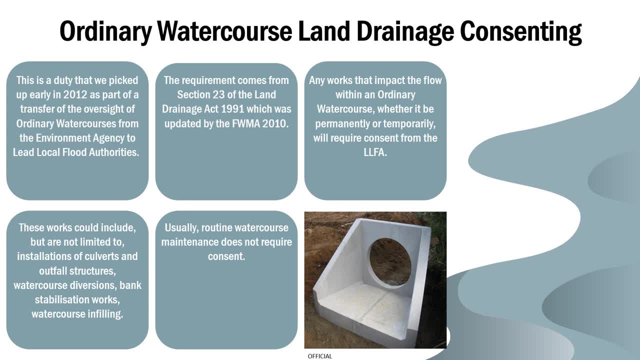 the flow rate can be represented from the header of the report on the slide to make a change that can be applied along the entire flood and flood management act. http//wwwlta-watercourseorguk. that will show you some of the can be implemented policies for flood control. 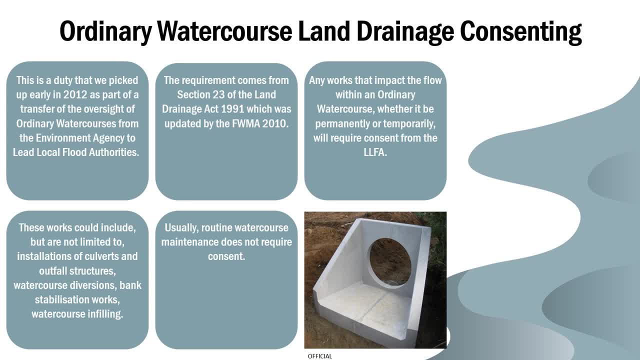 and the wind flow of the flood management act 2010.. the flood management act 2010 sacrifice water costs andDERWALDS could include, but are not limited to, available on our website. The LNFA aims to carry out community engagement work and aims. 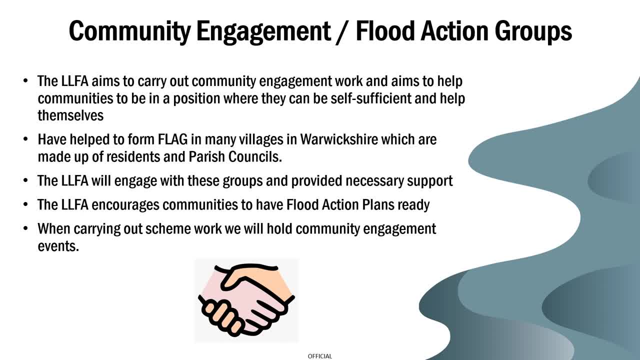 to help communities to be in a position where they can be self-sufficient and help themselves to better deal with flood risk. We have helped to form flood action groups in many villages in Warwickshire which are made up of residents and parish councils. The LNFA will engage. 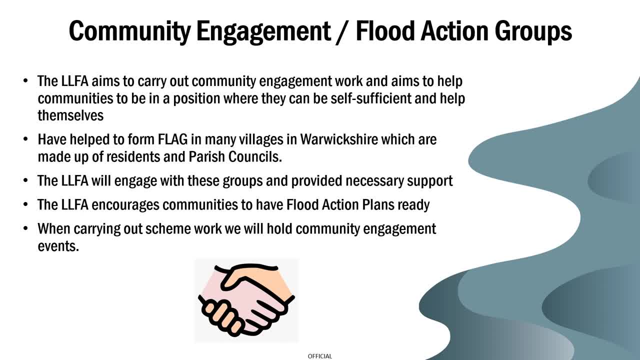 with these groups and provide necessary support, such as organising multi-agency meetings with partners to discuss issues within the village, offering training if it is deemed appropriate, and offering advice on what to do before, during and after a flood event. The LNFA also encourages communities to have flood action plans ready which help to improve resilience. 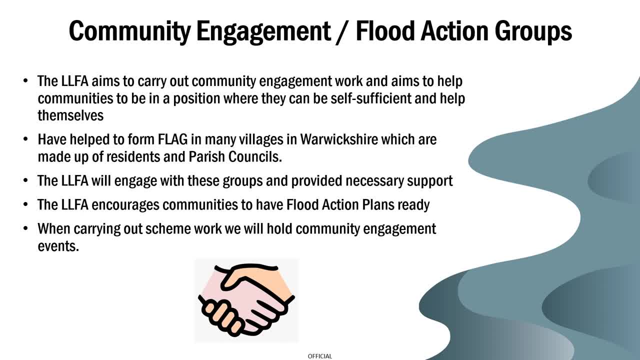 and reduce the risk of flooding. These will also be looked at by our internal CSW Resilience team When carrying out scheme work. we will also hold community engagement events to showcase the proposal to the community, gauge the level of interest and support the community. We will also hold community engagement events. 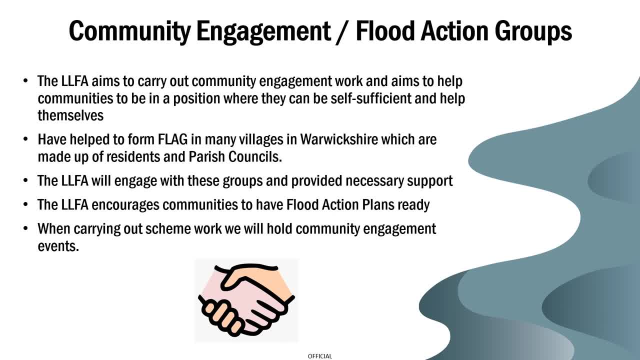 to showcase the proposal to the community, gauge the level of interest and support the community. We will also hold community engagement events to showcase the level of interest and answer questions and take on board any feedback communities may have, as, after all, communities have a lot of local knowledge which can be very useful to us. 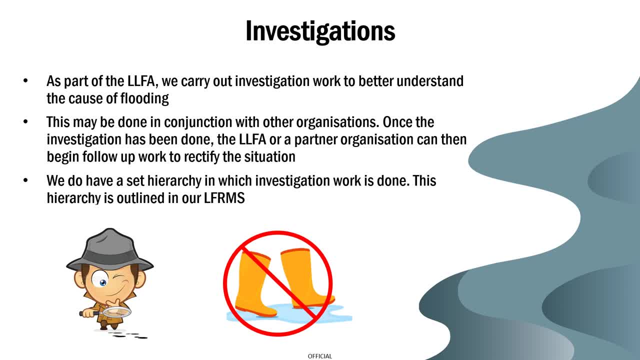 As part of our role as lead local flood authority for warwickshire, we carry out investigation work to better understand the causes of the flooding. This may be done in conjunction with other organisations, for example county highways, the Environment Agency or Seven Throne Water. Once the investigation has been done, the LNFA or report partner organisation. 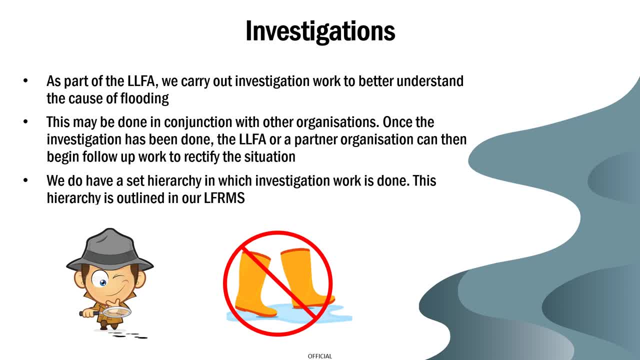 can then begin follow up work to rectify the situation. We do have a set hierarchy in which investigation work is done in, and this hierarchy is outlined in our local flood management strategy or previously in this video. Depending on the size of the flood event, certain incidences of flooding, such as external, 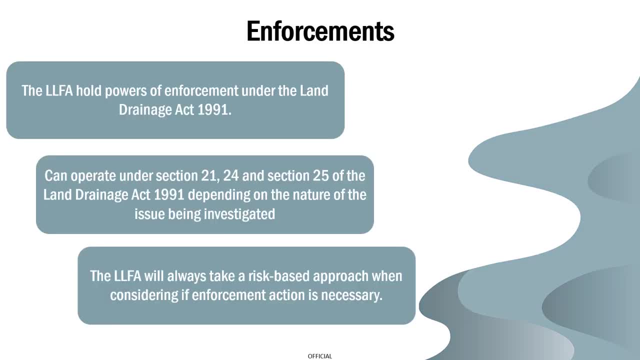 flooding may not be investigated. Under the Land Drainage Act 1991, lead local flood authorities hold powers of enforcement where it is deemed necessary to rectify the causes of flooding. Under this Act, we can operate under a number of different sections, but the most common 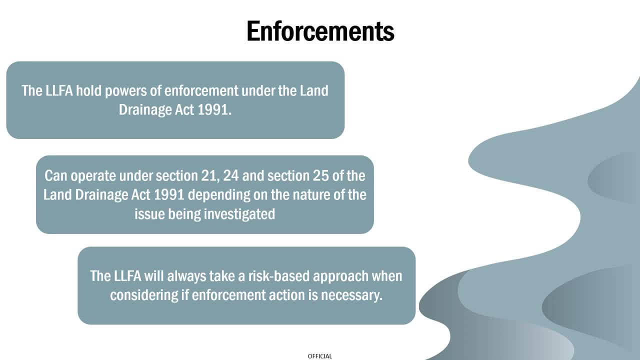 sections we use are section 21,, 24 and 25.. Section 21 of the Land Drainage Act gives us powers to enforce if landowners do not carry out the necessary repair works through a watercourse. Section 24 gives us powers to enforce if the cause of flooding is due to unconsented works. 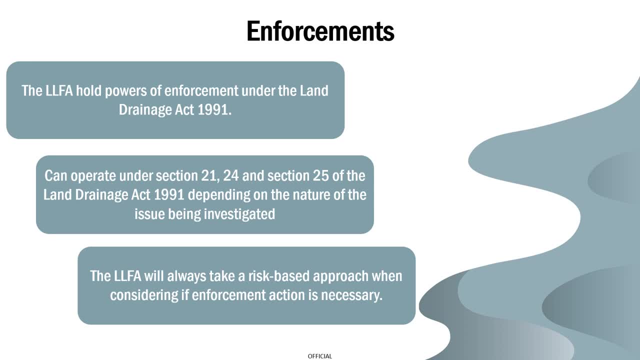 and section 25 gives us powers to enforce if the cause of flooding is due to unconstitutional watercourse. The LNFA will always take a risk based approach when considering if enforcement action is necessary and will always try to work with the relevant parties to rectify the situation. 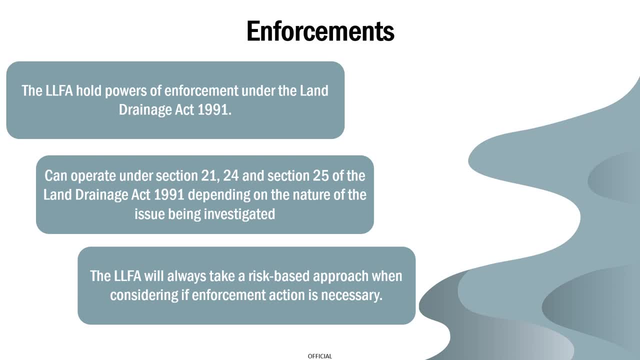 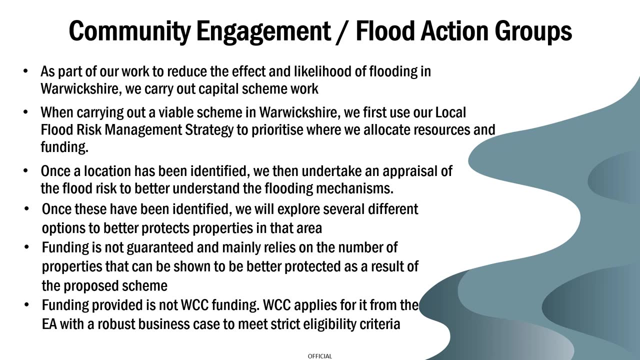 prior to enforcement action being taken if it is deemed appropriate As part of our work to reduce the effect and likelihood of flooding. in Warwickshire we carry out capital scheme work in locations deemed to be at high risk of flooding. If a scheme is deemed viable in Warwickshire, we first use our local flood management strategy. 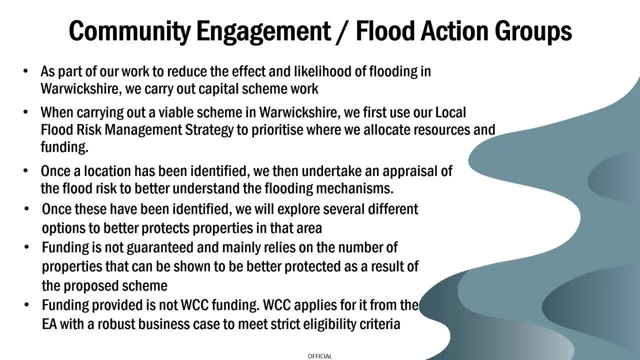 and then we use our local flood management strategy to ensure that the flood management is carried out. Once the location has been identified, we then undertake an appraisal of the associated flood risk to better understand the flooding mechanisms in the area. This may be done in the form of a hydraulic model, as an example.